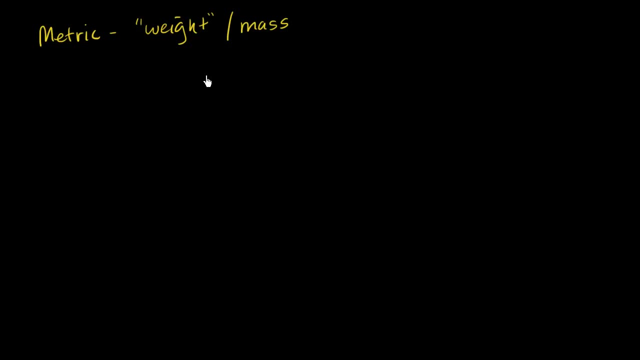 we'll see later on in our scientific careers that weight and mass are not the same thing. They are related. Mass, you could view, is how much stuff there is. How much substance does an object have? How hard is it to change the velocity of an object While weight is? 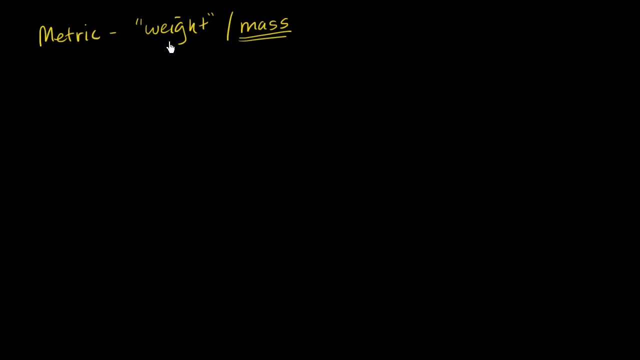 what's the force that gravity is pulling down on that object? Now, in everyday life, if we're just on the same planet or the same part of the planet, if something has more mass, it's going to have more weight, And if something has more weight, it's going to have more mass. 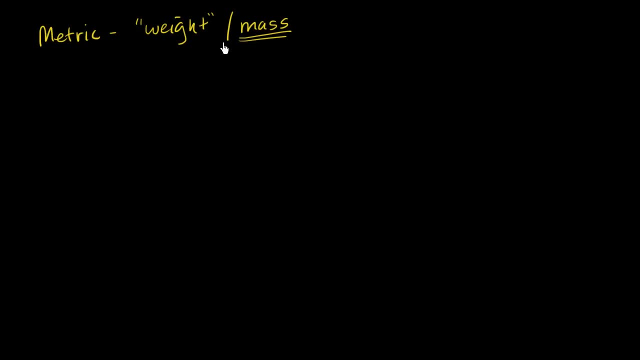 And that's why, in everyday language, these words are often interchanged. Later on we'll see that these mean different things For the sake of this video, because we're really just getting ourselves warmed up with some of these things we're going to talk about. 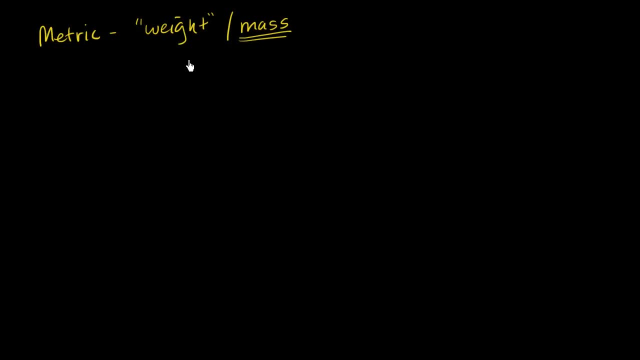 some of these units. I will use these interchangeably. I'll use them in kind of the everyday language sense, not in the technical physics sense of the word. So in the metric system when people talk about measuring relatively light things, they will often use the gram And 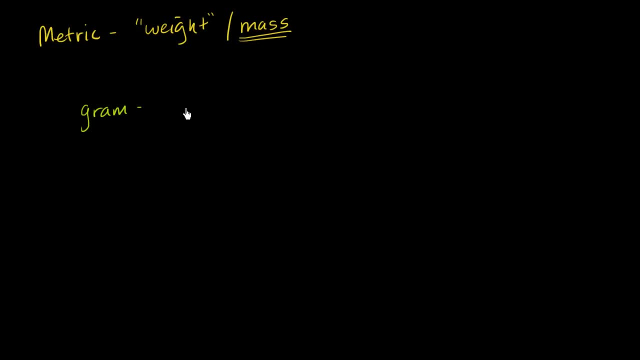 to get a sense of things that weigh a gram. one example is a paper clip. Your average size paper clip would weigh about a gram. A stick of chewing gum- not even the whole pack of chewing gum, A stick of chewing gum would weigh about a gram. A dollar bill would weigh about a gram. 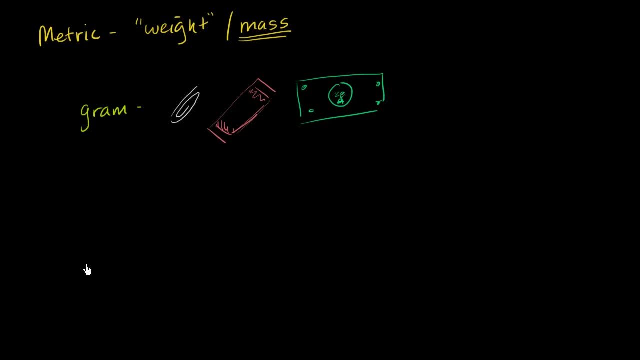 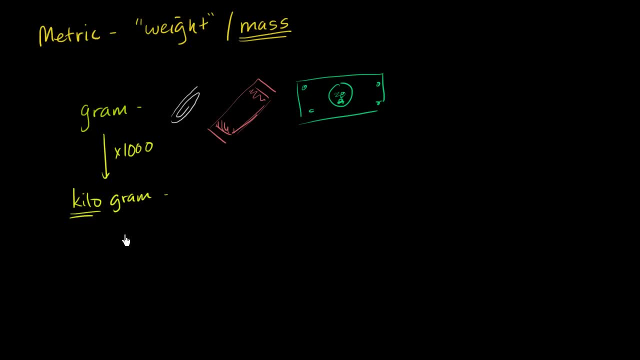 Kilo. Kilo A 1000. This means 1,000 grams, And if you want to think about how much that represents, well, many people will measure their weight in terms of kilograms. So I, for example, weigh about 70 kilograms And I'm 5'9" and I'm about average build and 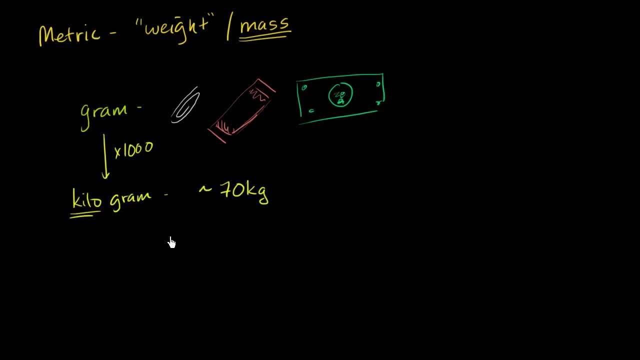 I weigh about 70 kilograms. If you want to imagine what eight kilogram is like, imagine taking a liter of fluid. So if you were a liter of water, you'd hear how wide it is in liters. and I'm saying, when you take the unattended gram you're basically losing 20 of that. 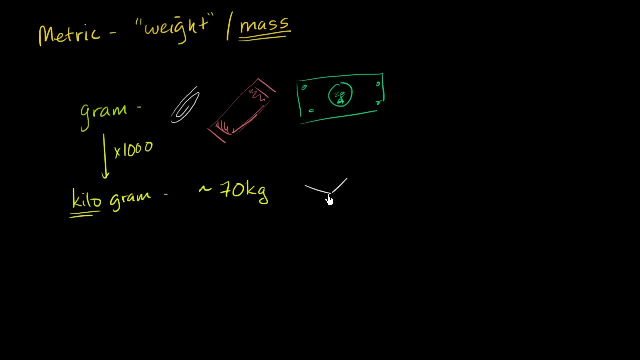 So you're literally losing an draws. So just make use of that so that it might mean that you're having issues when you're pulling it apart. So if you took a liter of water and a liter you could imagine as a 10 centimeter deep cube, 10 centimeters wide. 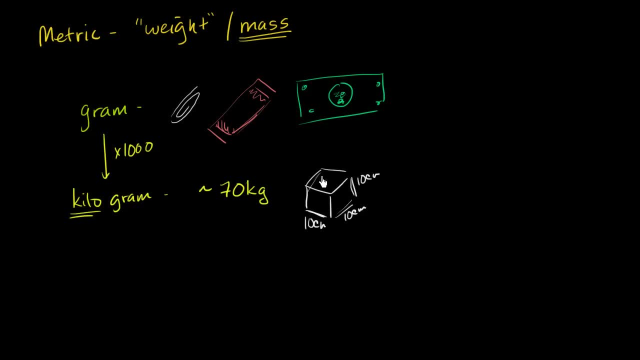 and 10 centimeters high. if you fill this up with water, the weight of that thing is going to be one kilogram, And things I know you're not used to walking around with one liter cubes of water. Another way of thinking about it if you go to the supermarket. 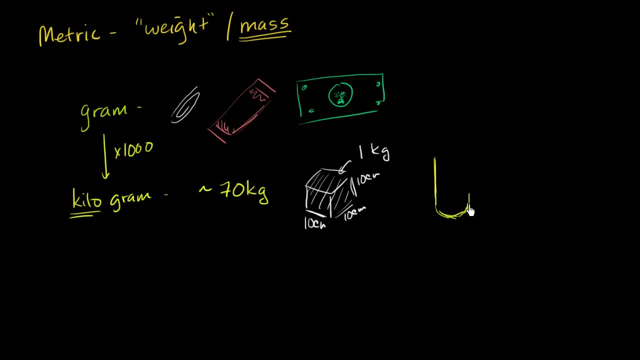 and you were to buy a two liter of soda. you were to buy a two liter of soda, and sometimes you can buy two liters of other things as well of water. whatever, if you buy a two liter, two liter of soda is going to weigh, is going to weigh. 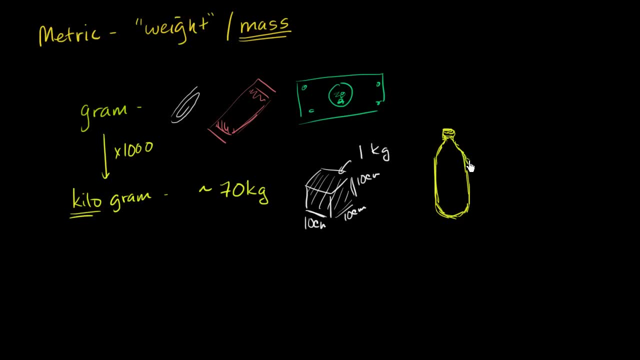 well, actually two liters of water in particular is going to weigh soda. it has other things in it, so you can't be as precise with the weight, but two liters of water, I should say, are going to weigh exactly two kilograms. 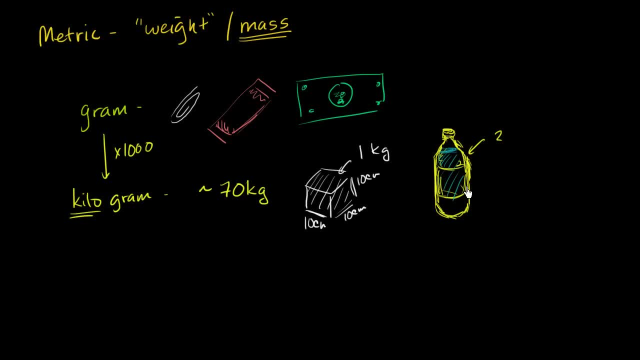 If we don't, we're just talking about two kilograms. We're just talking about two kilograms. We're not talking about the water itself, We're not talking about the container, But if you want to get a rough sense for how much weight, 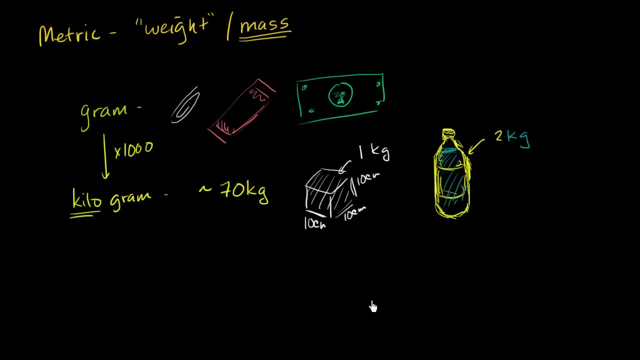 that is. that's going to be two kilograms. So if you're measuring, you know human scale, size things, reasonable size quantities of fluid objects around this scale. kilogram makes a lot more sense If you measure these very light things. 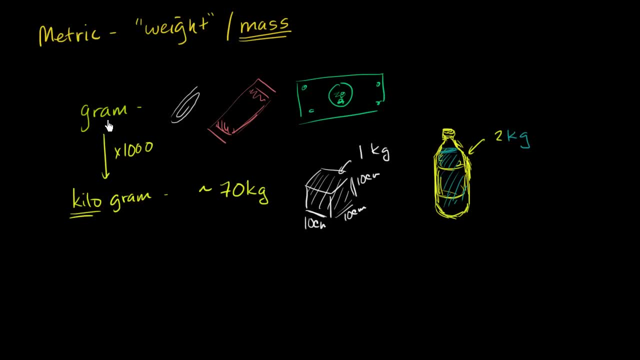 you're talking about. you're talking about a gram. If you want to get really precise, this might be more in things of if you're doing you know a drug dosage and you need to be very, very, very precise, then you will sometimes see people. 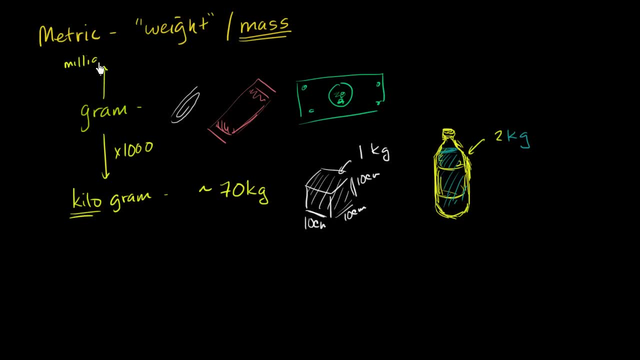 go to the milligram. the milligram, But you can imagine, a milligram is one thousandth, one thousandth of a gram, And so one thousandth the weight of a dollar bill, or one thousandth the weight of a paperclip. 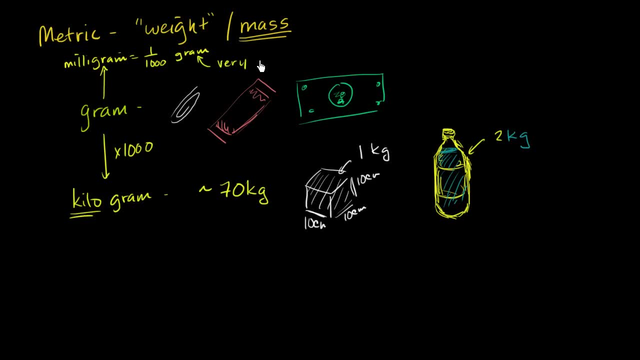 this is very, very, very, very small, So this usually doesn't come into play in our everyday life.